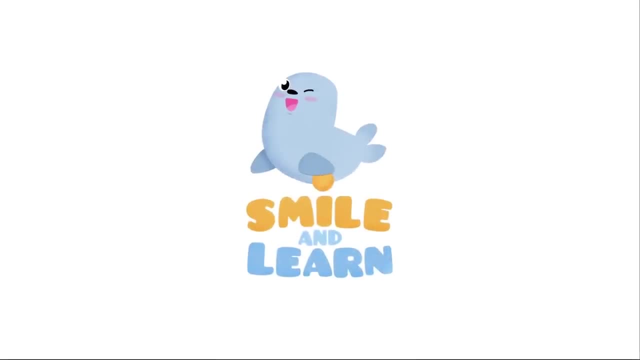 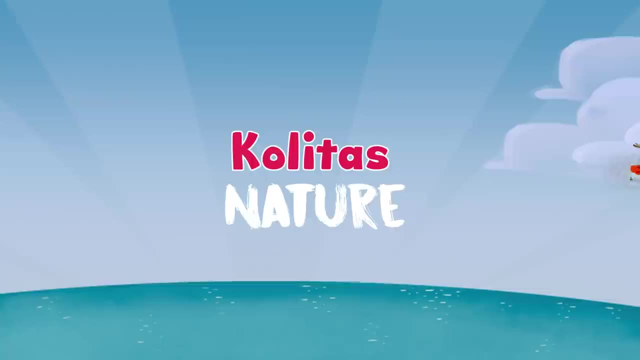 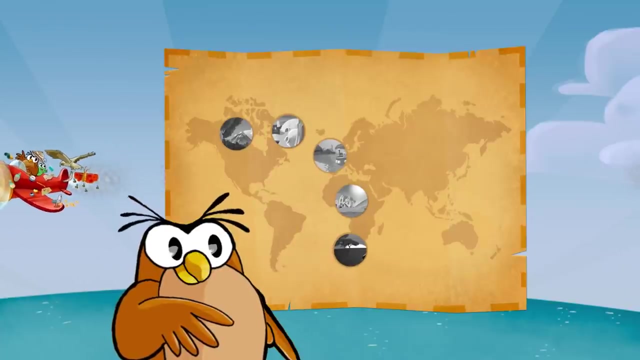 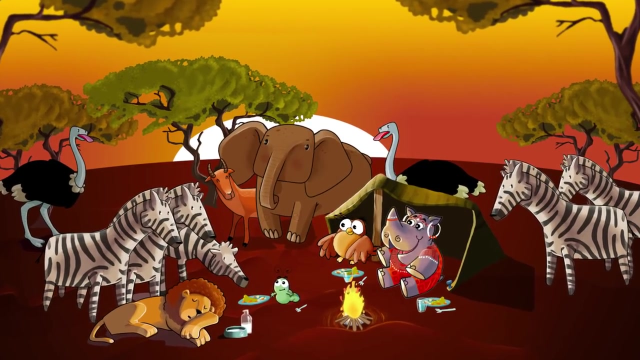 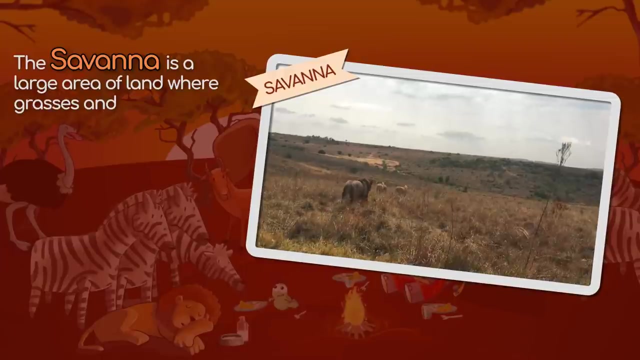 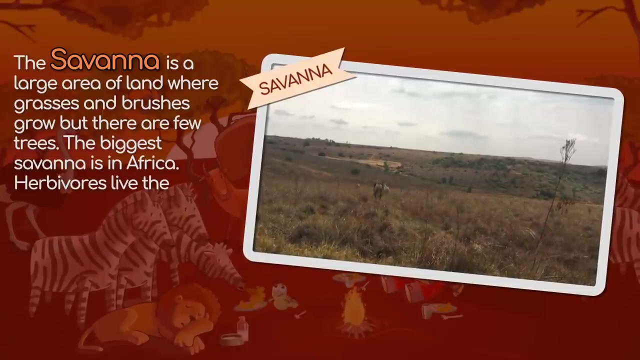 Welcome to Galita's Nature. Today, we're going to learn about the savanna ecosystem. The savanna is a large area of land where grasses and bushes grow, but there are few trees. The biggest savanna is in Africa. Herbivores live there that eat grasses, and also large. 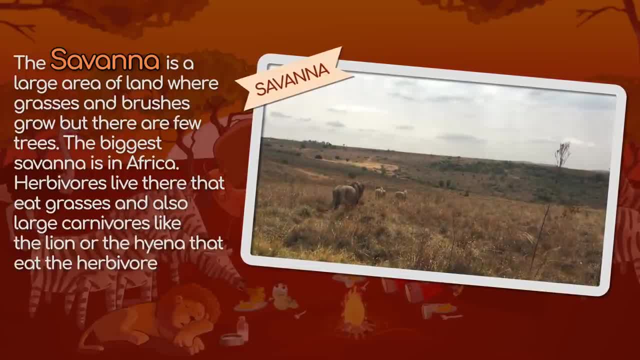 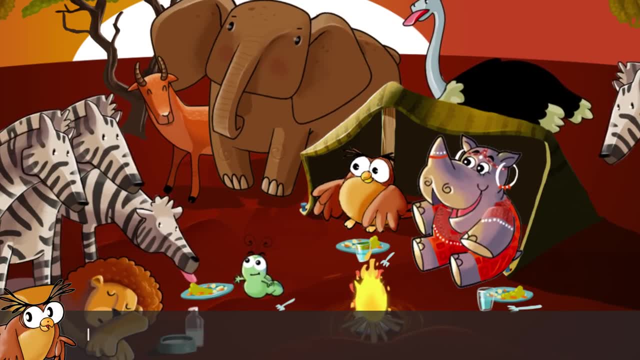 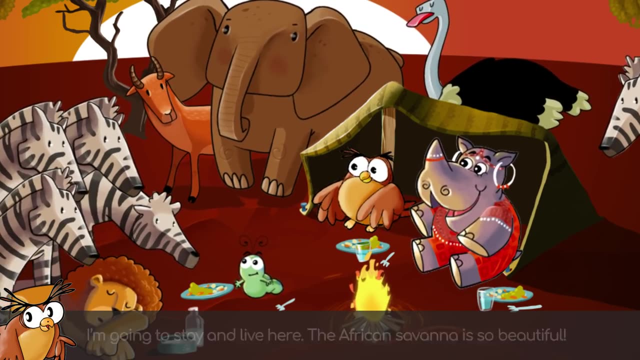 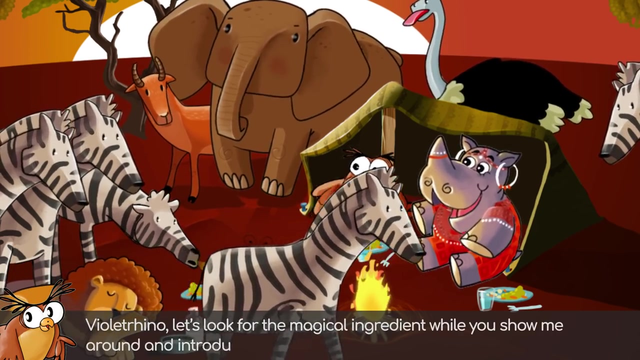 carnivores like the lion and the hyena that eat the herbivores. I'm going to stay and live here. The African savanna is so beautiful. I'm going to stay and live here. The African savanna is so beautiful. Violet Rhino, let's look for the magical ingredient while you show me around and introduce. 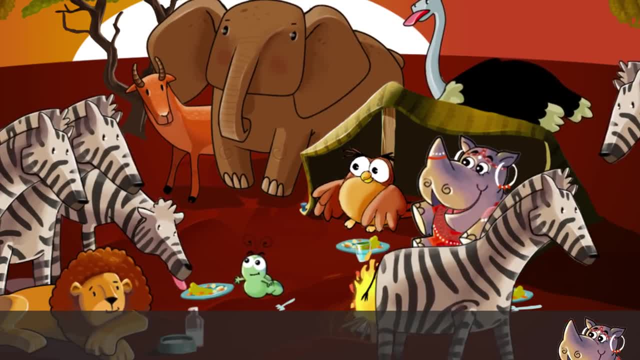 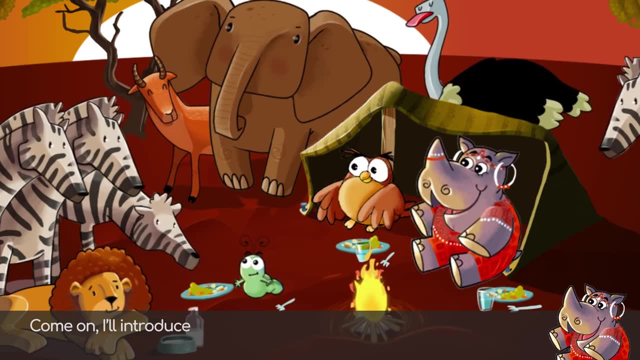 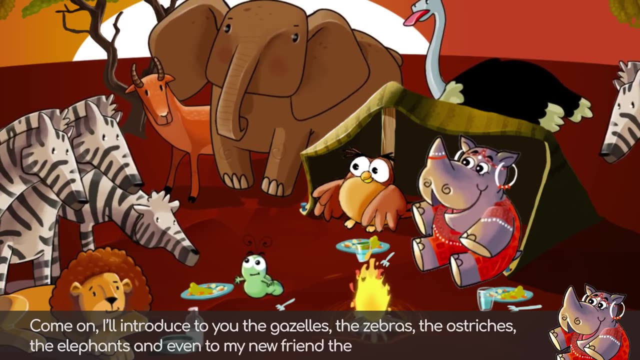 me to your new friends, Guys. did you know that the fastest animals on the planet live in the savanna? Come on, I'll introduce you to the gazelles, the zebras, the ostriches, the elephants, and even to my new friend, the lion. Don't be afraid, but don't get too close either. 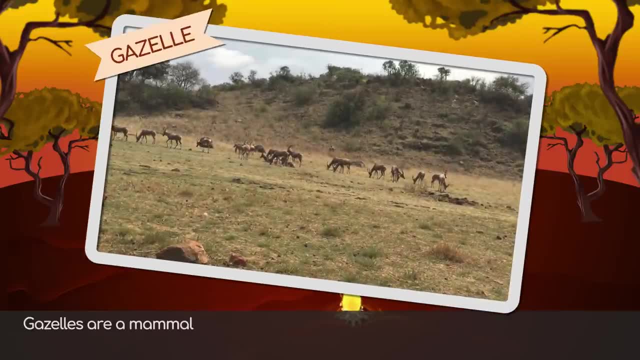 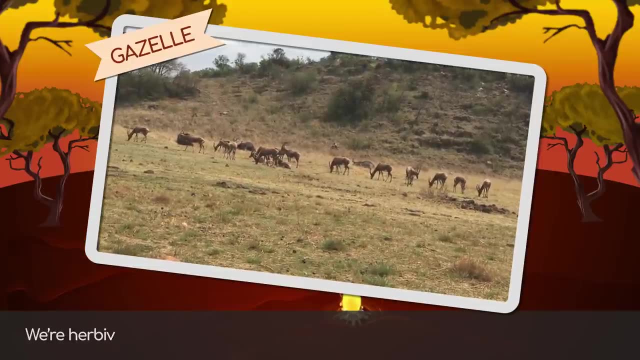 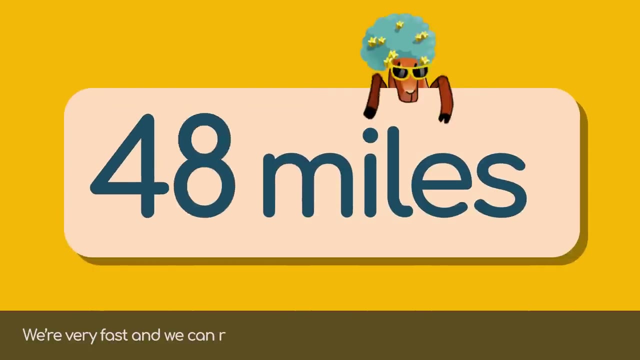 Gazelles are a mammal from the antelope family. We live on the African savannas in large groups. We're herbivores, since we eat branches, grasses, seeds and leaves. We're very fast and we can run up to 60 miles per hour. 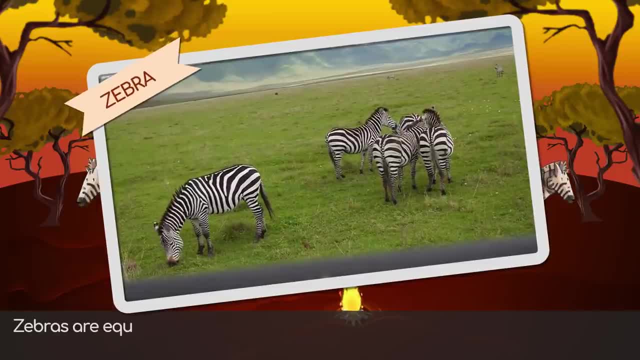 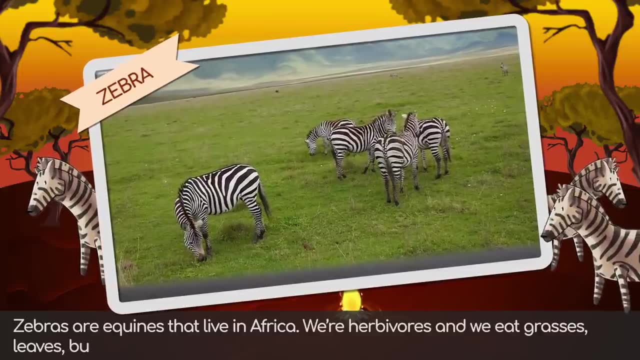 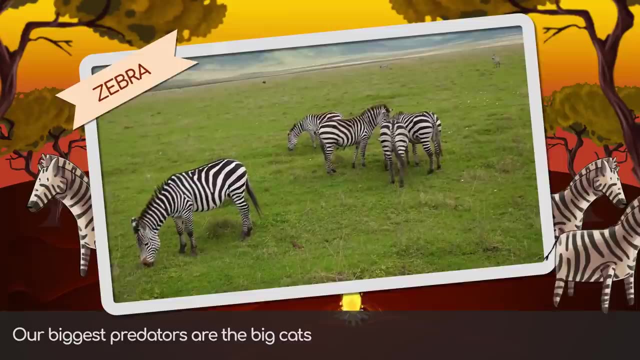 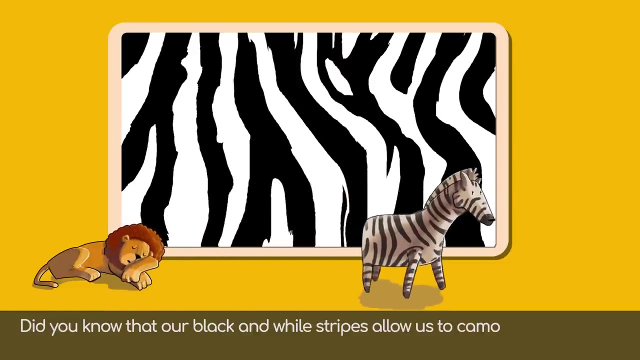 Zebras or equines that live in Africa. We're herbivores and we eat grasses, leaves, bush stems, branches and bark. Our biggest predators are the big cats who live on the savanna. Did you know that our black and white stripes allow us to camouflage ourselves, to hide from? 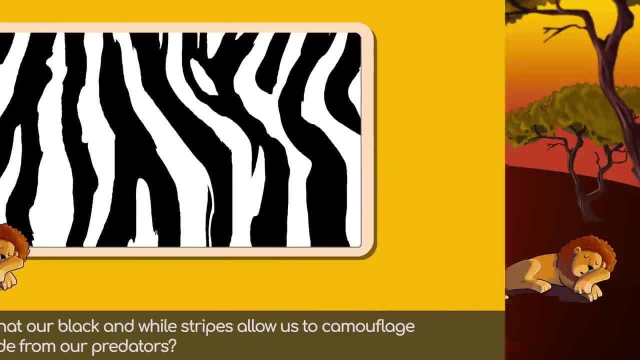 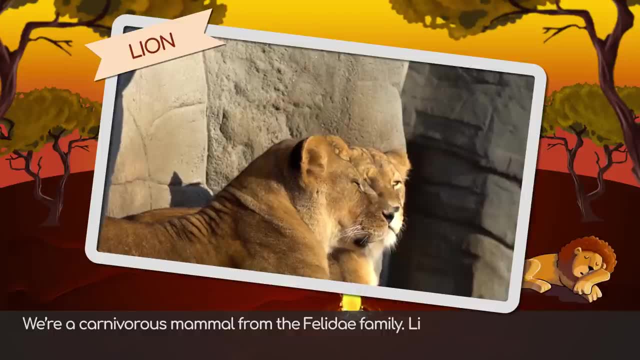 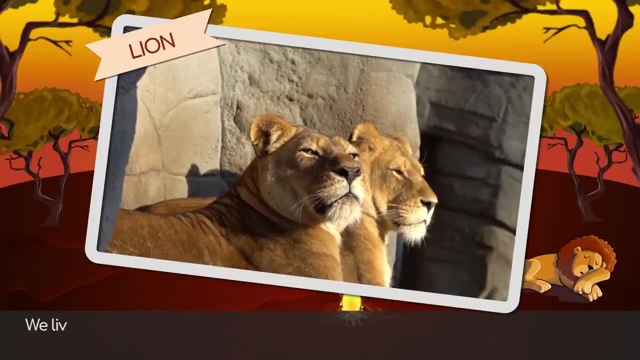 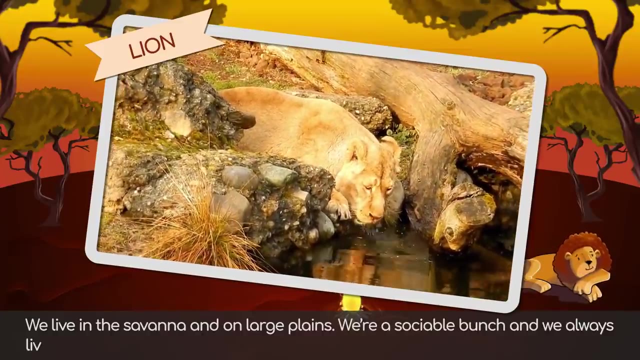 our predators. We are a carnivorous mammal from the Felidae family. Lions can hunt big animals like zebras, buffalos and noobs. We live in the savanna and on large plains. We're a sociable bunch and we always live.